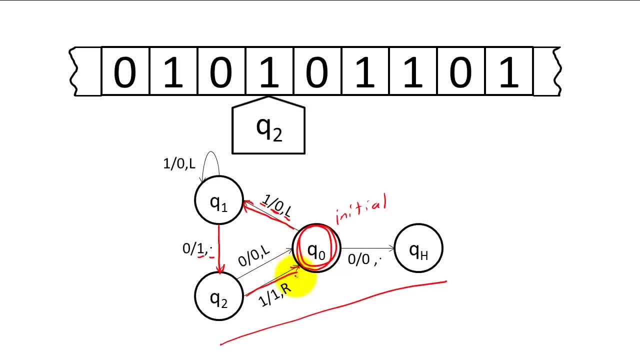 Our state diagram tells us to transition back to our initial state, change the current cell value to 1,, which it already is, and move the head to the right. Finally, since our state is the initial state and our current cell's value is 0,, we transition to the halting state. 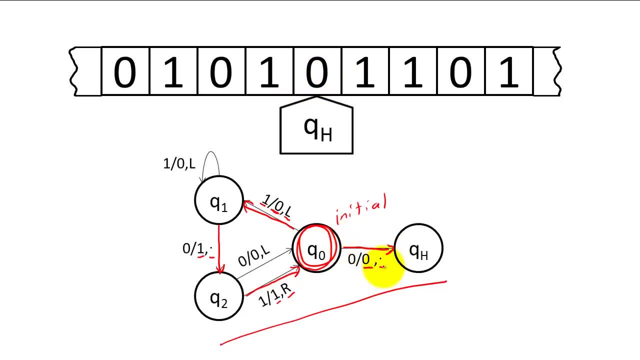 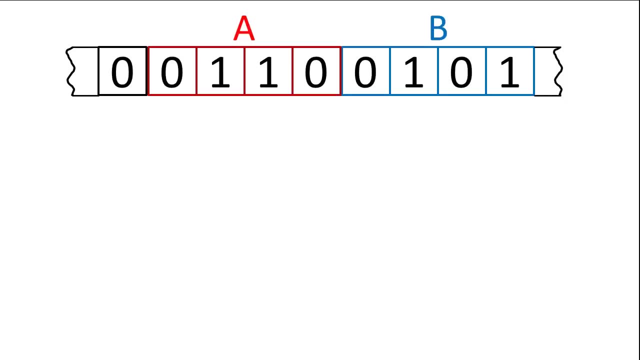 Change the value in the cell to 0 and keep the head in the same place. The halt state is another critical state that every Turing machine needs. Without the halting state, the machine will keep looping forever and never complete its programmed task. Let's take a step back and look at the Turing machine at a more abstract level. 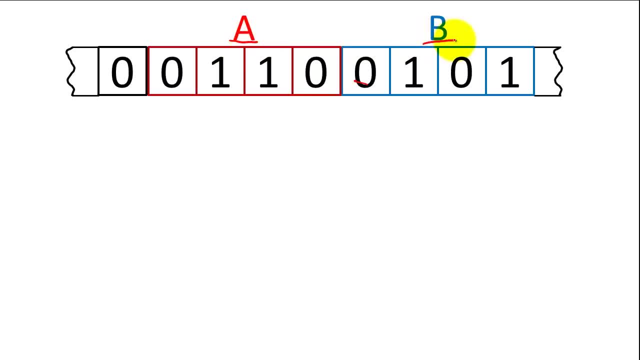 Suppose you have a tape with two values, a and b, stored on it. We could build a Turing machine that would perform the addition operation on a and b and store the summation back onto the tape. We would simply need to create a state machine that would control the Turing machine appropriately. 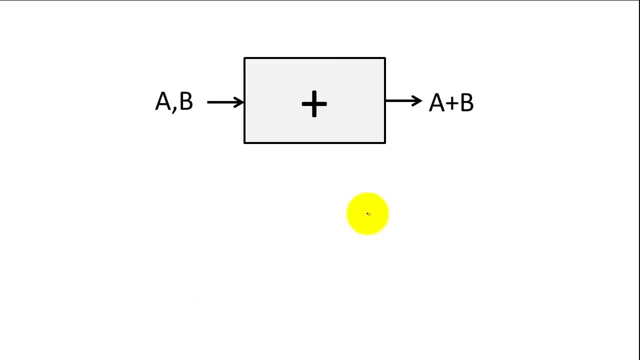 We could represent this type of system with a black box notation in which we show our inputs entering a black box and our output leaving it. We could then theoretically represent a machine to perform any legal computation, such as multiplication. More generally, we say that each Turing machine has inputs, outputs and a program p that describes its behavior. 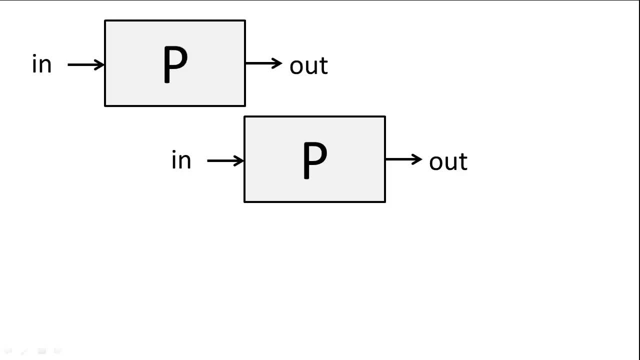 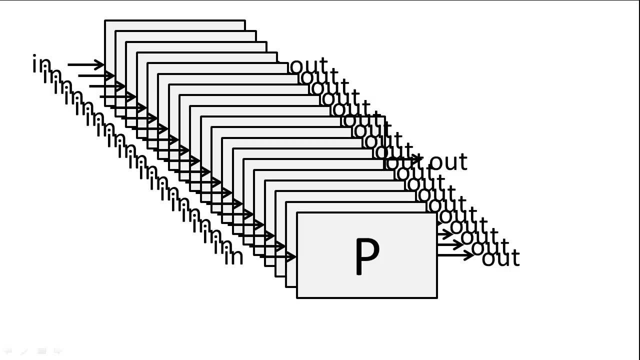 The problem with these types of Turing machines is that we need to create a new Turing machine for every operation we want to perform. As you will learn later, creating hardware is much more expensive than writing software, So creating a new Turing machine for every operation is intolerable. 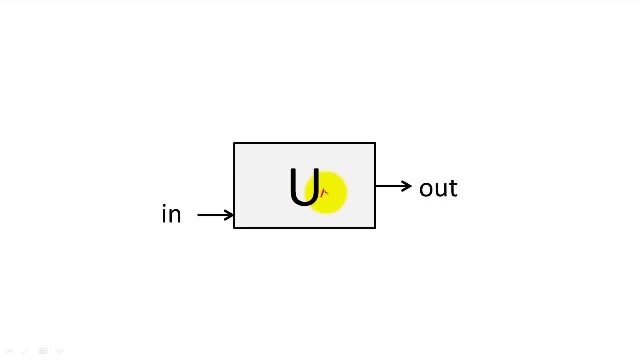 So Turing invented the Universal Turing Machine. This machine had a basic state machine that could be programmed by a machine description, p, so that to the external user the Universal Turing machine would behave exactly like a regular Turing machine that was programmed to do p. So that to the external user the Universal Turing machine would behave exactly like a regular Turing machine that was programmed to do p.